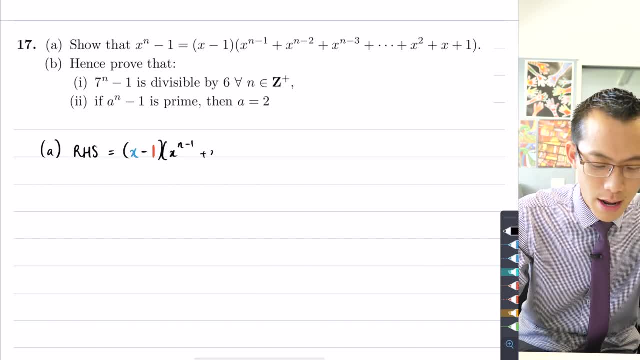 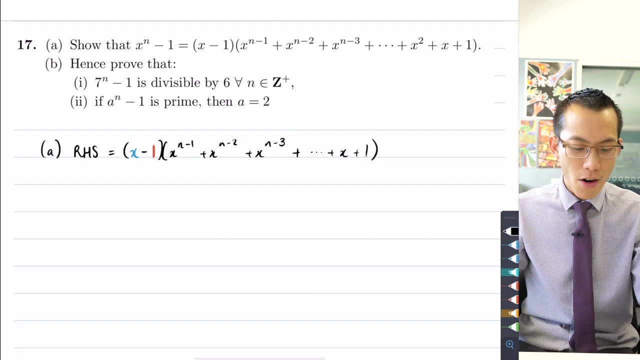 distribute all of these terms, So x to the n minus 1,, x to the n minus 2, establish the pattern with the third one: dot, dot, dot. I actually don't think I need to do the last three terms. I'm just going to do the last two. I think will do it. Alright, so I've got. 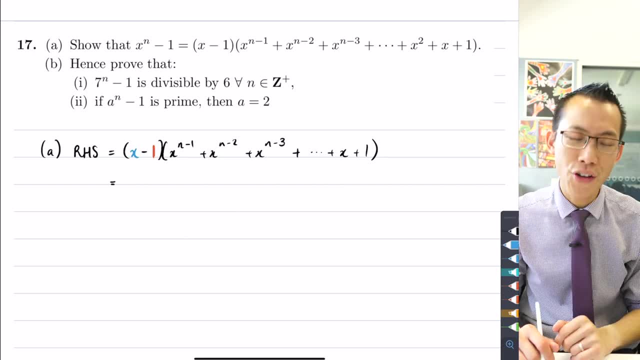 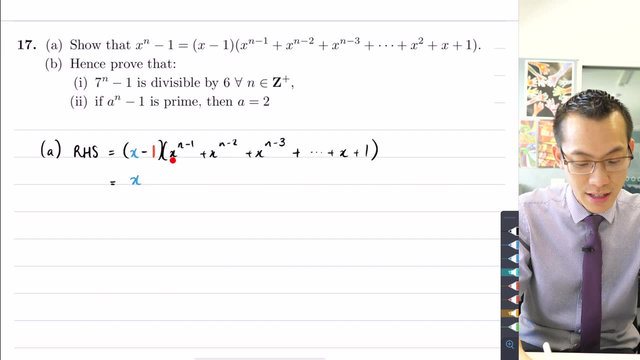 my algebraic sort of brackets ready to go, let's start expanding. I'm going to do the x's first. So when I multiply this first First term here by x, this is x to the n minus 1 times x to the 1.. So we add the indices. 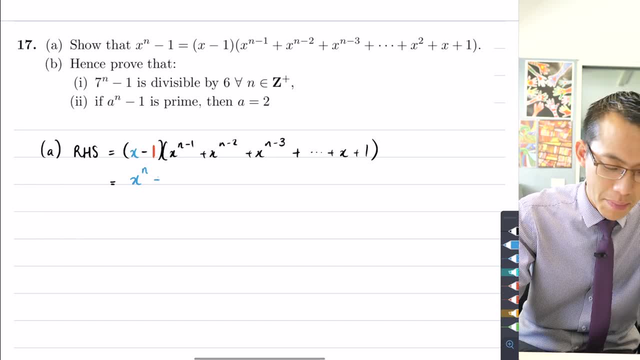 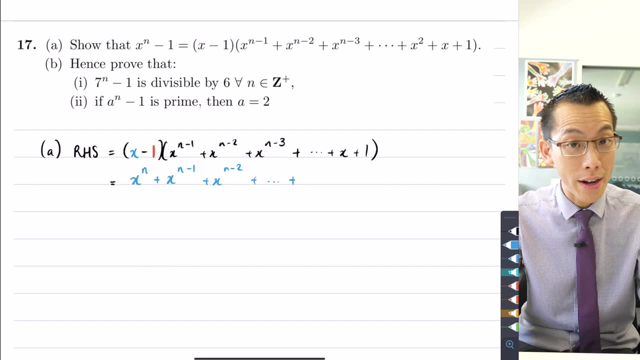 and we just get x to the n. The next one along is just 1 powered down, so it's x to the n minus 1 plus x to the n minus 2, and then so on. When I get to the end, that x turns into: 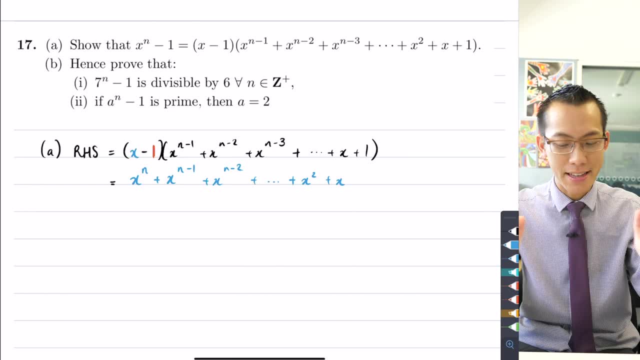 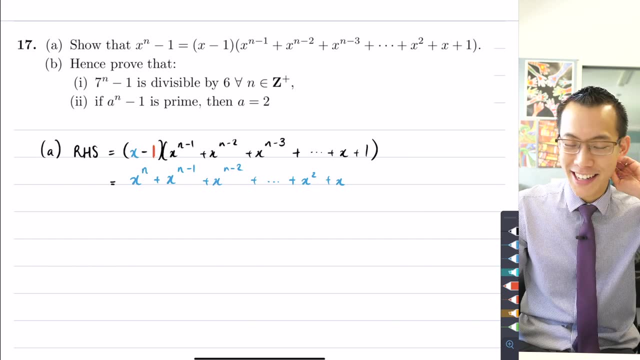 an x squared, and then the 1 turns into an x And that's it. I have distributed everything from the x's. Now I'm going to do the minus 1's, and they're even easier For reasons that you might recognise. 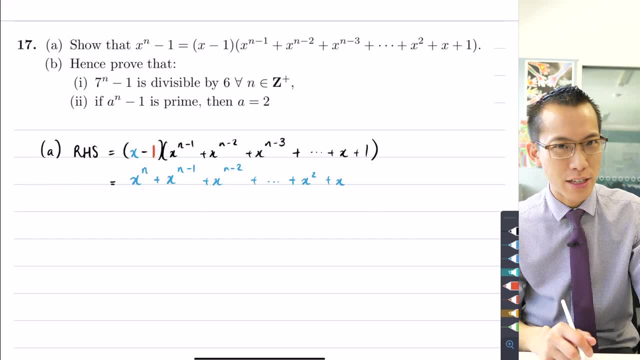 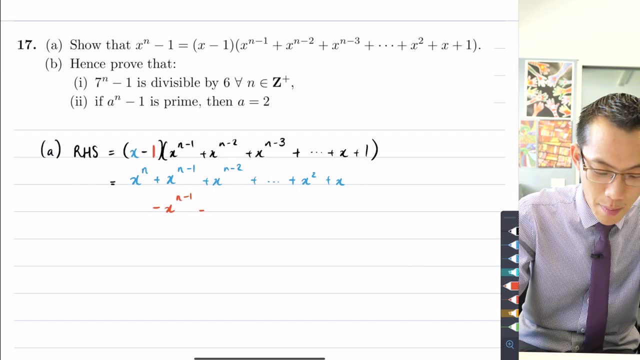 Before I even say it, I'm going to stagger these terms and move them one along, just to make some cancelling and collection of like terms easier in a second. So here we go: minus 1 minus x to the n minus 1 minus x to the n minus 2, minus x to the n minus 3, just to. 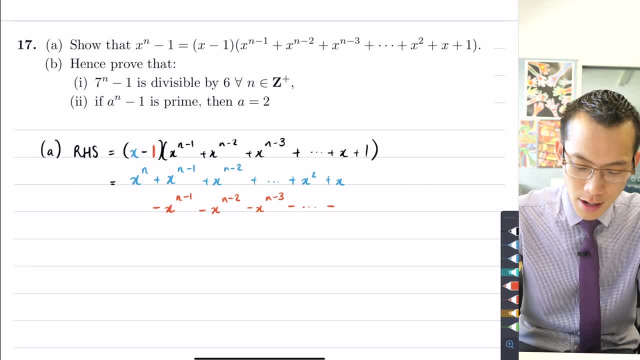 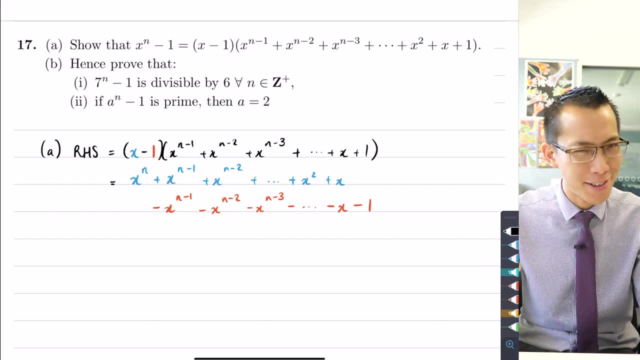 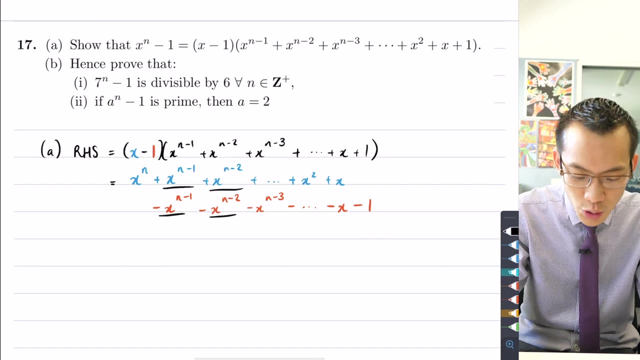 continue the pattern: minus dot, dot, dot, And then my last terms are x and 1, and that's it. So what do I see here? Well, a whole lot of this is going to collapse and cancel with each other. My x to the n minus 1 terms, of course. cancel X to the n minus 2 terms. cancel This x to. 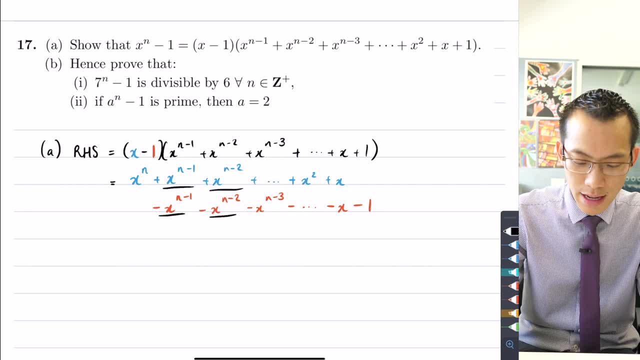 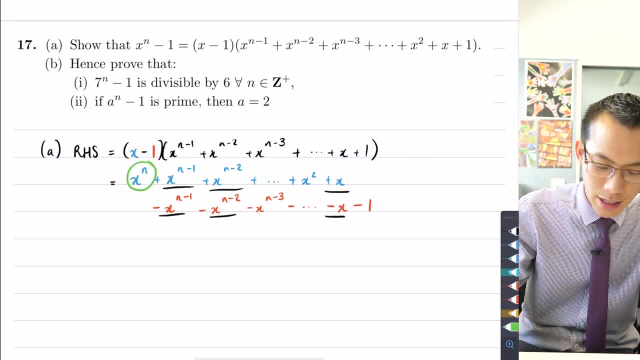 the n minus 3 would cancel, if I've written all the terms there. But you also see the, and the same thing with the x squared. But then, lastly, you see these x's cancel, which leave you with these terms here: x to the n and the minus 1, which is of course what I 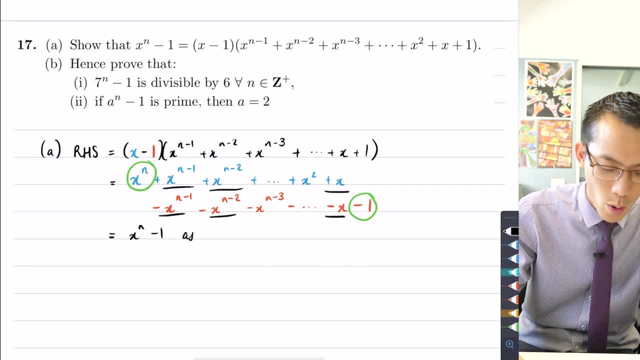 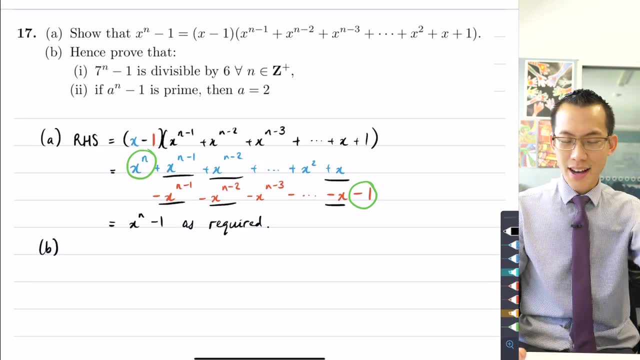 was after: So x to the n minus 1, as required. Okay, Wonderful. How am I going to use these for part b? Well, you're going to see, these are some of those questions where there's very little working actually, but a lot of thinking. 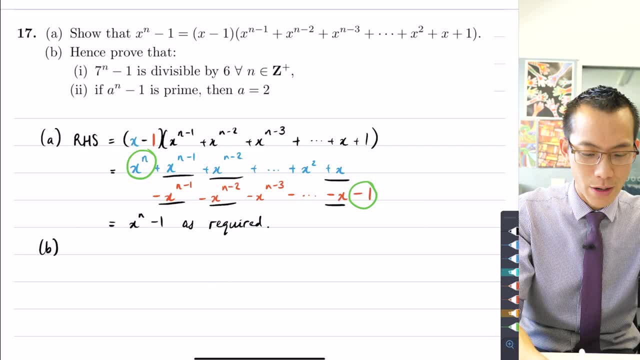 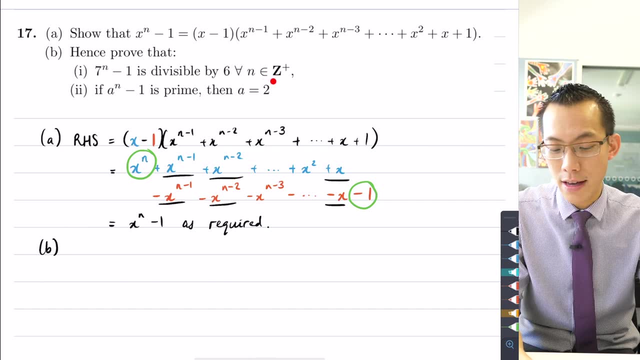 that's involved underneath them. so what's the first one we want to have a look at here? prove that s 7 to the n minus 1 is divisible by 6 for all values of n, where n is a positive integer. because how does this work? before we actually do the proof, i just want to note like what are: 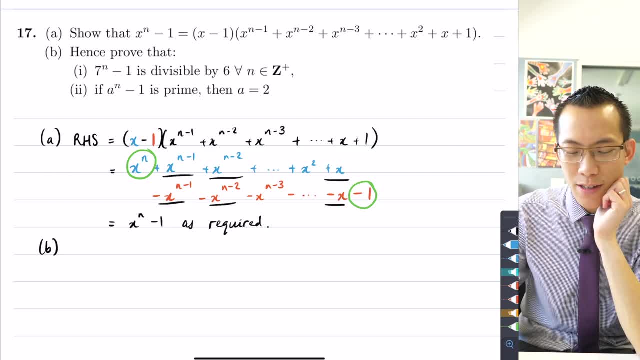 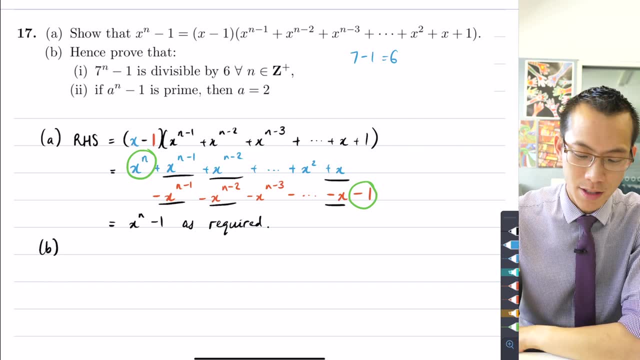 these numbers, 7 to the n minus 1. well, 7 to the 1 minus 1. 7 is 7 to the 1, rather is 7 minus 1, which equals 6. obviously. that's divisible by 6. what's the next one? 49 minus 1 is 48. that's divisible by. 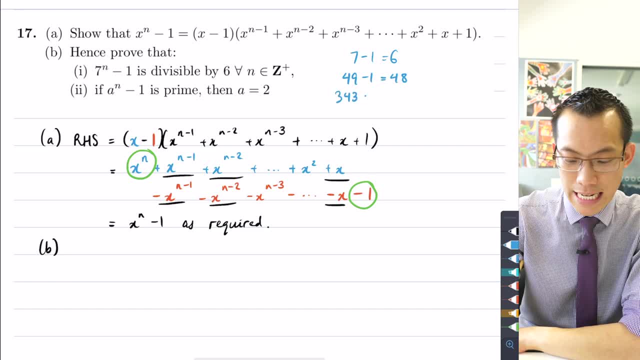 6, great. the next one along is 343. take away 1 um 342, sure, i guess. so 300 is divisible by 6, 42 is divisible by 6. looks good. and the last one i know off the top of my head is 2401. you subtract. 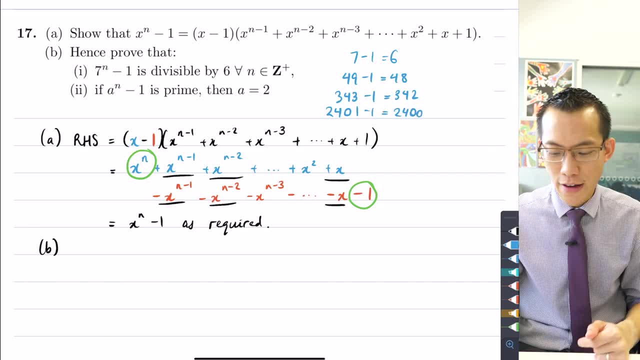 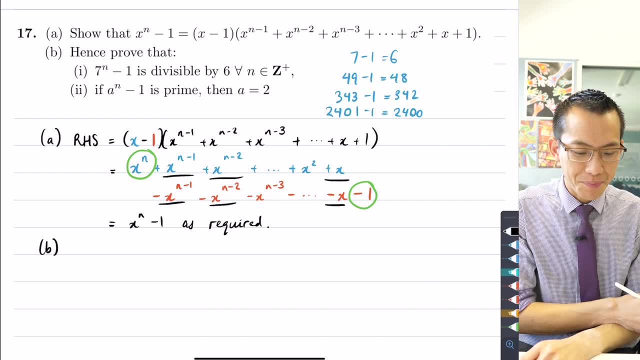 1 and you get 2400, which, again fairly uncontroversially, is divisible by 6. so it's nice, we can look at this, and we can look at this, and we can look at this, and we can look at this- at least see it works. how do we prove it? what i'm going to do, simply, is to use part a for part one. 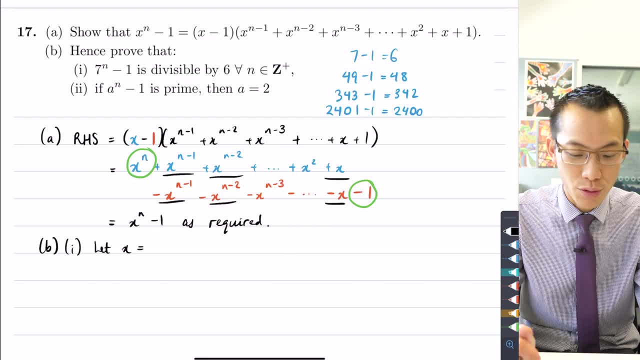 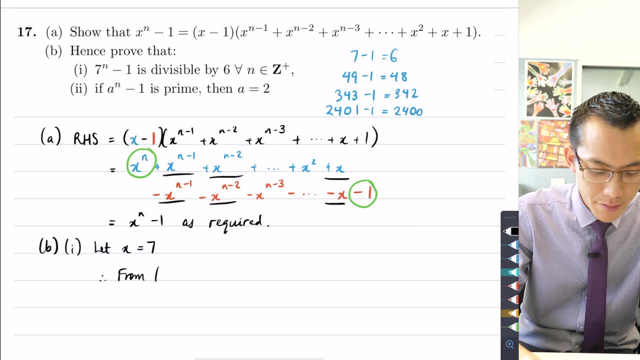 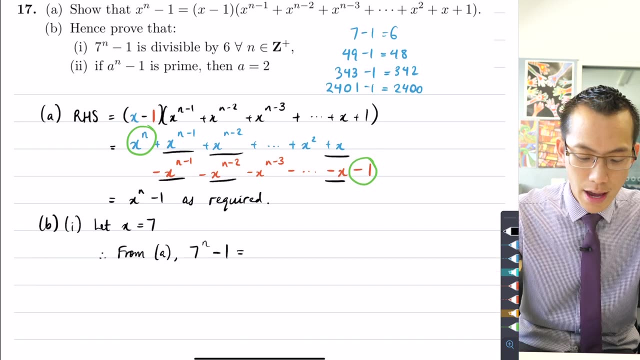 i'm going to say: well, let's let x take on a value that's appropriate to this question and fairly obviously it's 7. so if x equals 7, therefore from part a, i can say 7 to the n minus 1, which is remember. the thing i want to prove is: is divisible by 6 is just equal to, and i'm just going to use 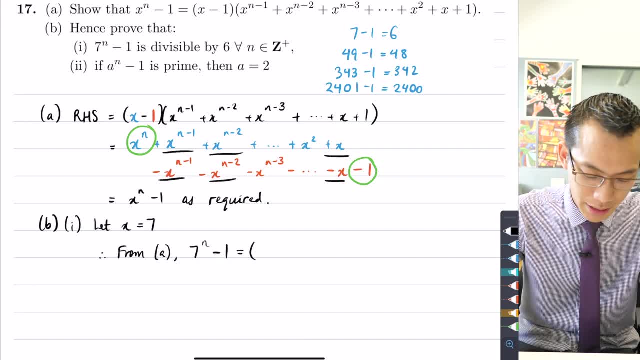 i'm just going to quote the result, substituting in 7 for x. so i get 7 minus 1, and then i've got 7 to the n minus 1, 7 to the n minus 2, uh, 7 to the n minus 3. establishes: 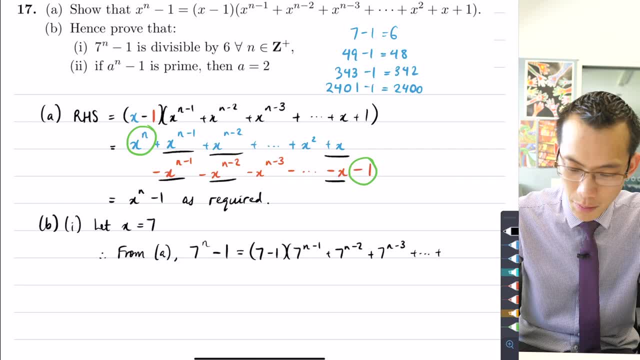 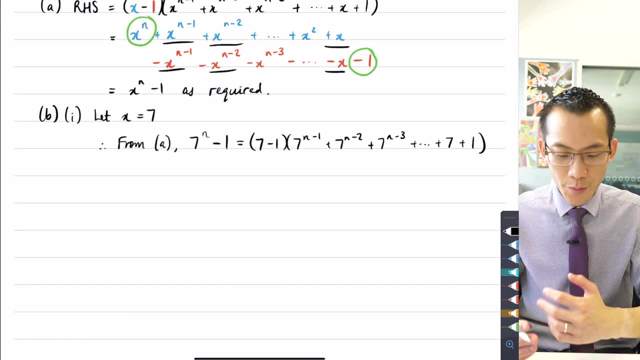 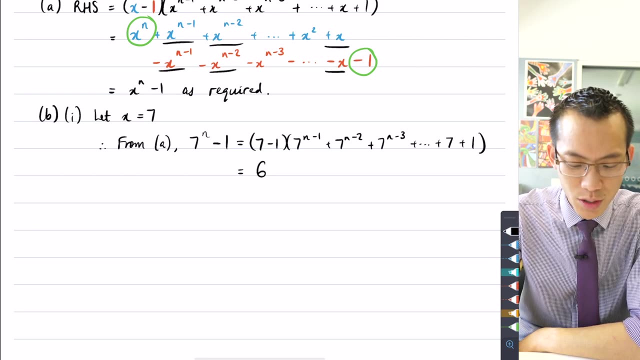 the platen: dot, dot, dot plus um. what am i going to have down the end there? uh, plus 7 plus 1. okay, now, what you can see here, hopefully, is that on the left hand side here, uh, or on the left part of the right hand side, uh, 7. take away 1. that's simply equal to 6, which is going to be very important to 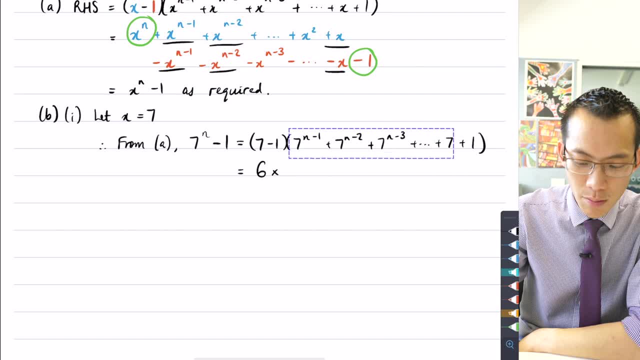 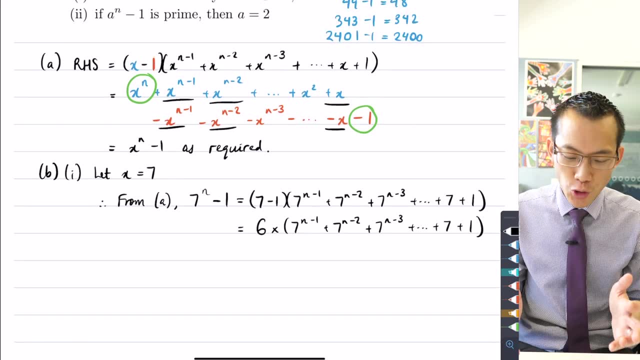 me in a second. that's multiplied by everything i've got here. so i'm going to take away 1 and i'm over here, and there's not much that i can do to simplify this now. where is the working involved next? well, you actually just need to think about this object that you've got over here. 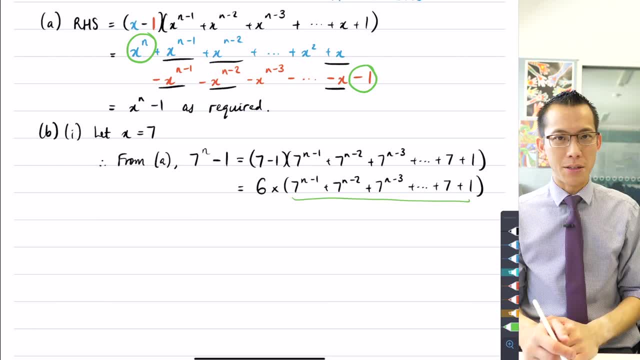 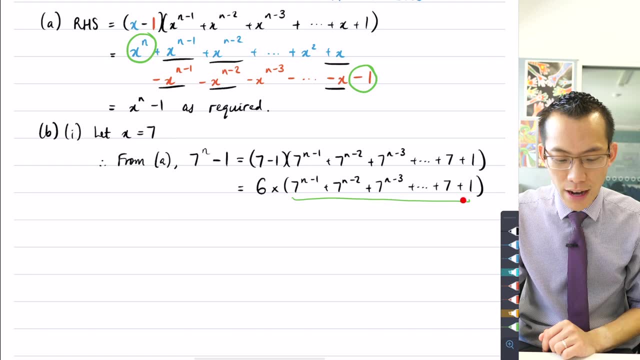 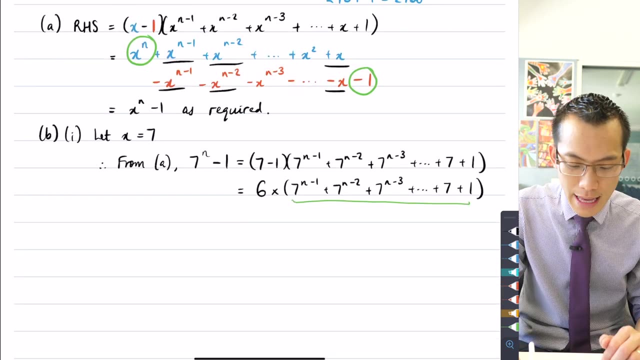 remember: what you've got here is going to be a series of integers, because even though we start with this 7 to the n minus 1, the lowest value that n can take is going to be- let's see here it's a positive integer, so n has to be equal to 1, which means that the 7 to the 1 minus. 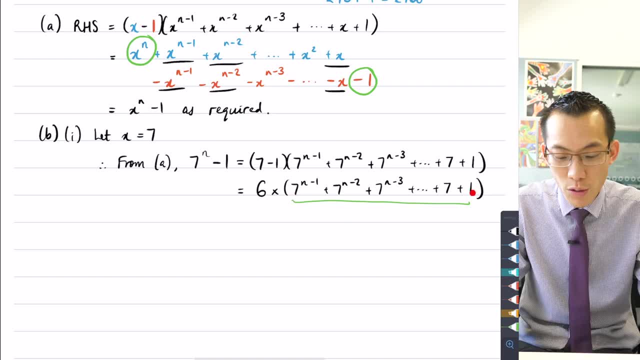 1 is 7 to the 0, which would be 1. there'd only be one term over there, and we saw that already it's 6 times 1, which is this first case over here. so even though there are several terms here, we've 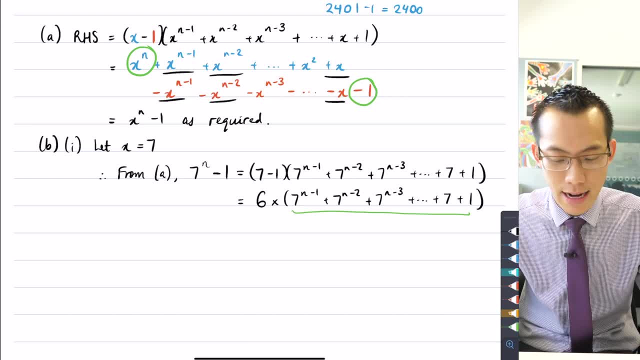 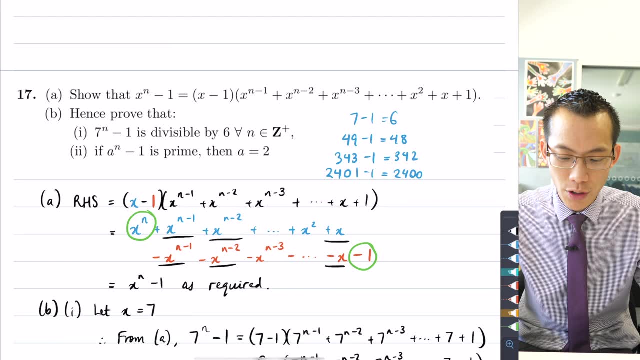 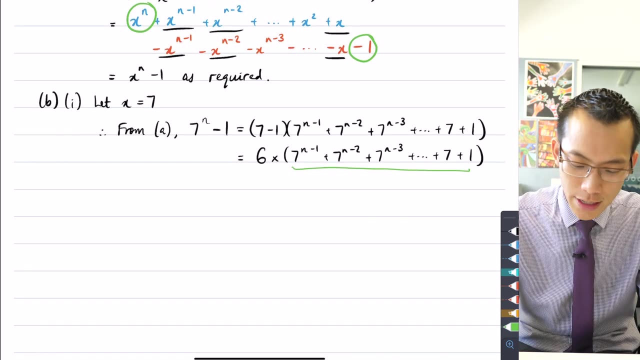 written this series just in case we need that many, depending on what n is, but the smallest this thing is going to get is 1. when you do the next one, it'll be 1 plus 7, which is 8, which is why we got 48 before, because that's 6 times 8. so what you can see here is a series of integers. this is a. 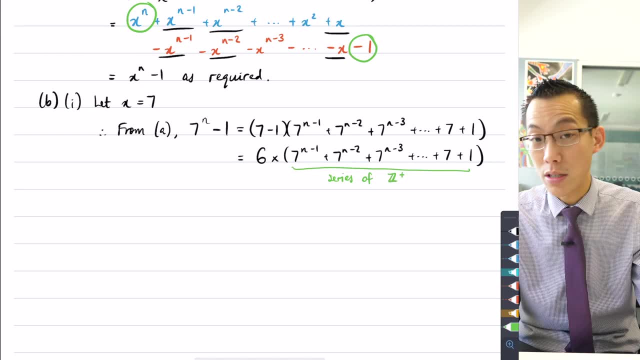 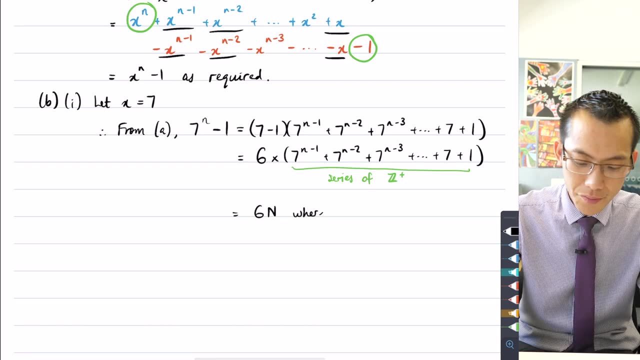 series of whole numbers, positive whole numbers as well. so therefore i've got 6 times n, where n equals 7 to the n minus 1. 7 to the n minus 2 is a capital n, which is a bit sneaky, but anyway, plus dot, dot, dot all the way to 1. so n is also a positive integer, and so if you have some number, 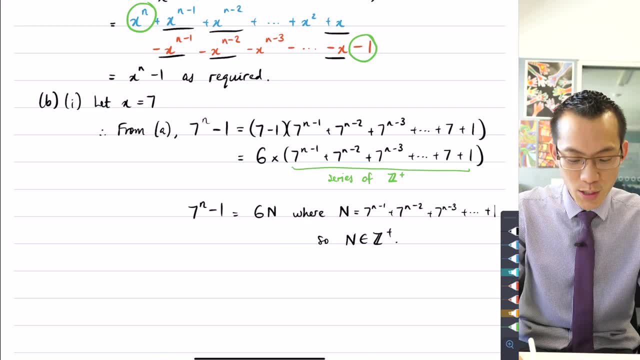 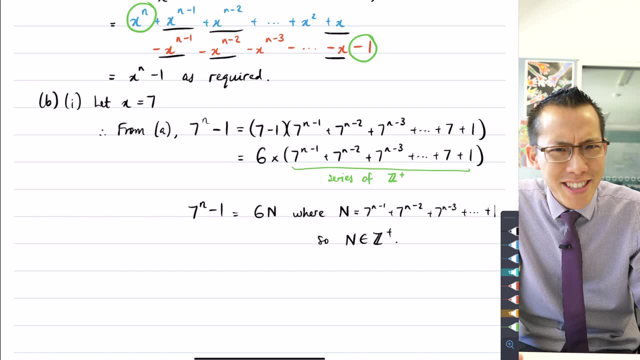 7 to the n minus 1, it can be rewritten as 6 times some other positive integer, which is the definition of divisibility by 6. so that's kind of it. there's not that much working to it. you just need to think carefully about the objects that. 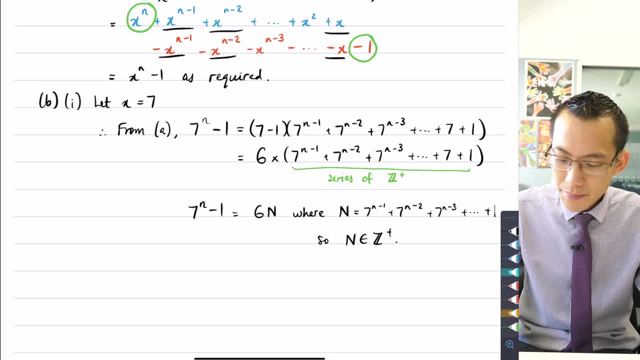 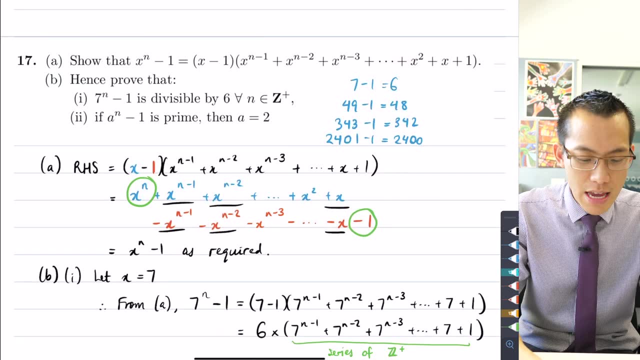 you've got and then do a little bit of cancelling. okay, now you're going to follow this theme. when you have a look at part 2, we're going to use the same algebraic result but to do something a little bit different. right? if 80 n minus 1 is prime, then a equals 2. this actually relates to a question. 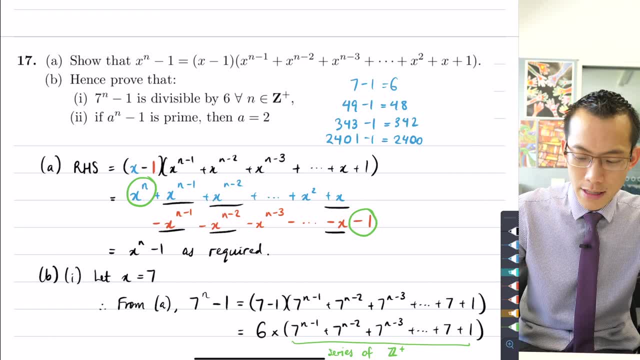 that we looked at earlier with the mersenne primes. these are the numbers of the form 2 to the n minus 1, where, in fact, if 2 to the n minus 1 is prime, we can know that n itself is prime, and this is the way we actually calculate all large prime numbers. 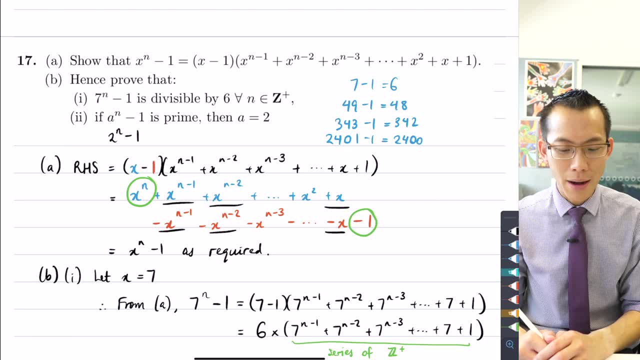 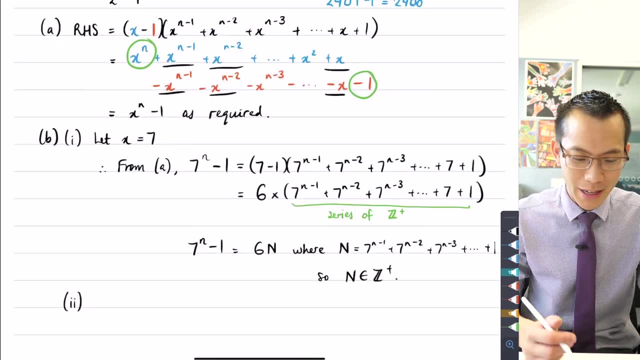 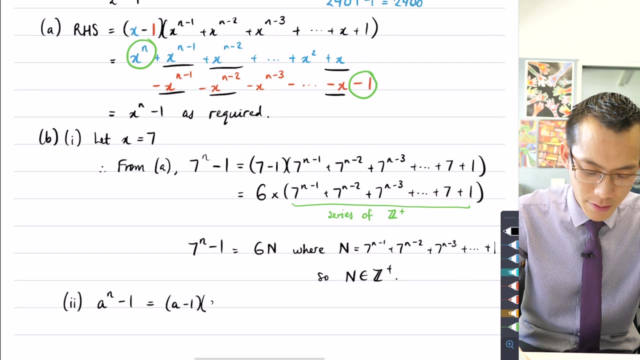 so how do i prove this? well, i'm going to start by using the result that we proved in part a, except instead of an x, i'm just going to write an a. so what do we get here? i'm going to write a to the n minus 1 is equal to a minus 1, and then here comes the rest of the. 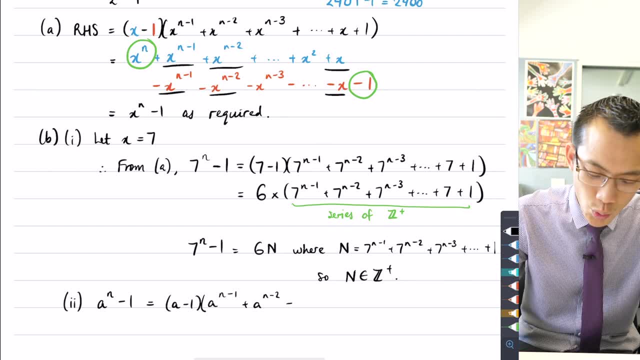 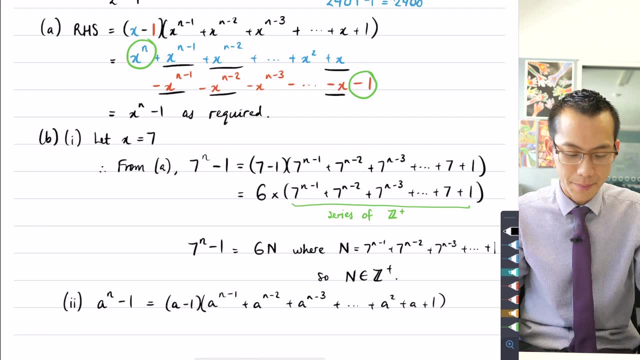 brackets: a to the n minus 1, a to the n minus 2, n minus 3. dot dot dot. where do we finish? a squared plus a plus one. and then the other thing they tell us is that a to the n minus 1 is prime. now, 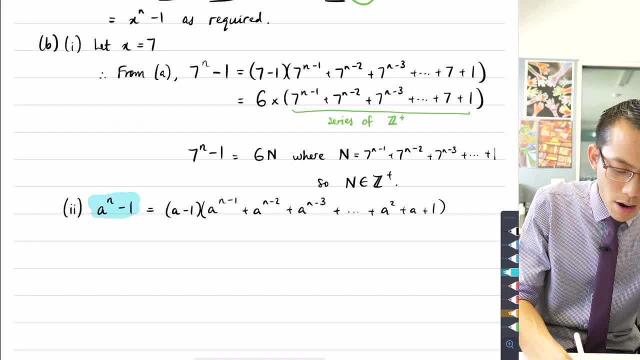 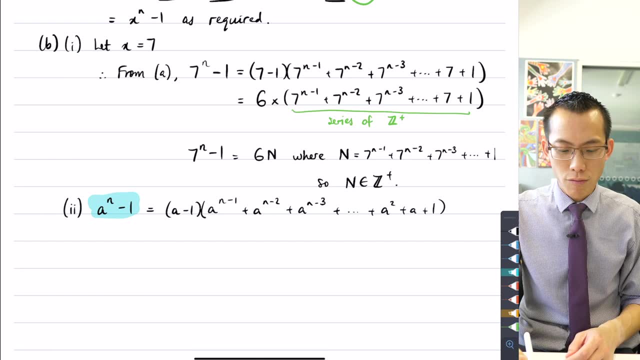 hold on a second. if a to the n minus 1 is prime, then it can't possibly be written as the product of two prime numbers. but that's an issue, right, because look, i've got this number over here being multiplied by this number over here. i should say not just because of the number, but because of the 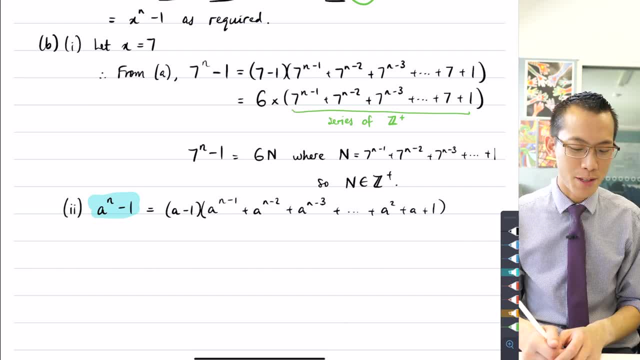 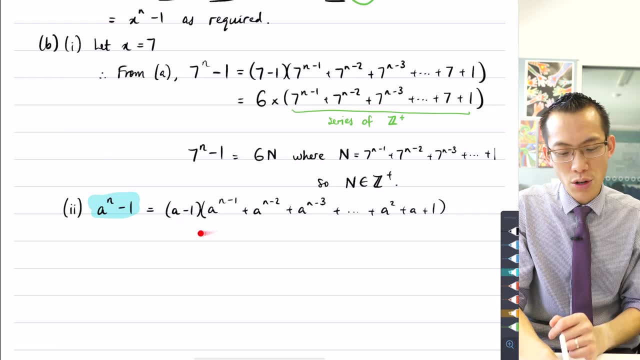 product of two prime numbers. you definitely can't be the product of two composite numbers, because then you're definitely not going to be prime. so if this is prime and it's expressed on the right hand side as the product of two positive integers, the only way this can work out is if one of the 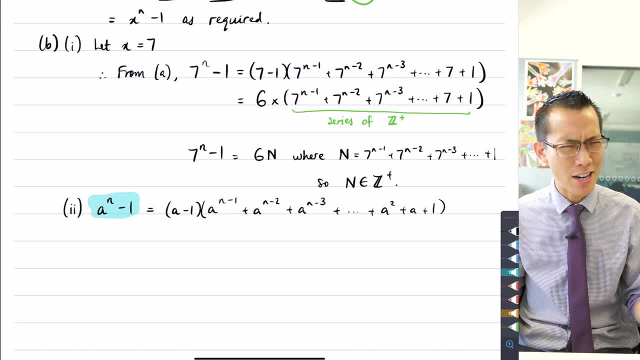 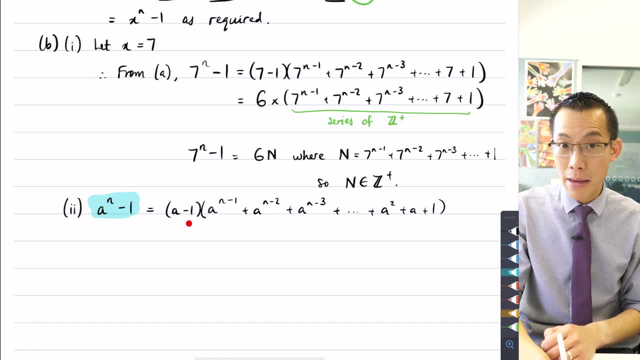 positive integers is equal to one right. think about this right. if i want the product of two positive integers to give me a prime number, those two positive integers better be one and a prime number. if they're both positive, then i'm going to have a positive number, and if they're both positive. 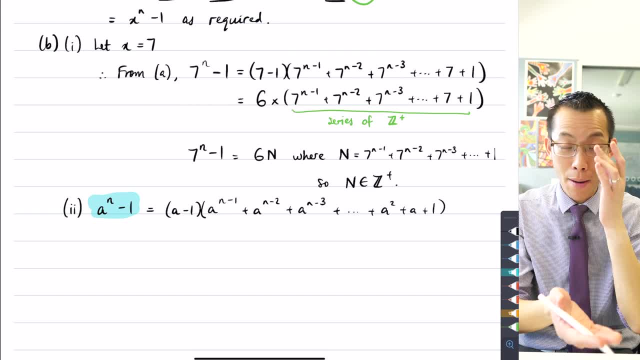 they're both prime you. you don't get a prime number at the end as a product, if they're, if neither of them is prime, then you're already in trouble. so one and a prime that will do it. and the reason why i'm highlighting that this has to be the other non-one number is that you start with one and then 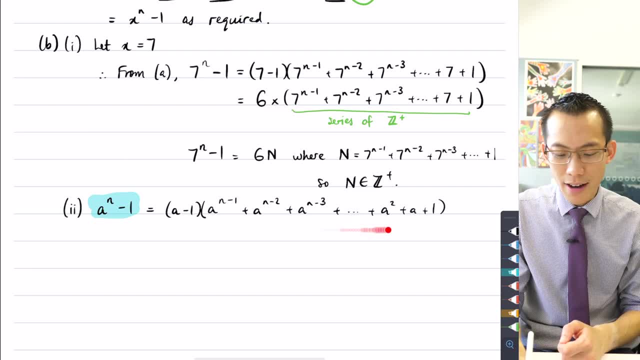 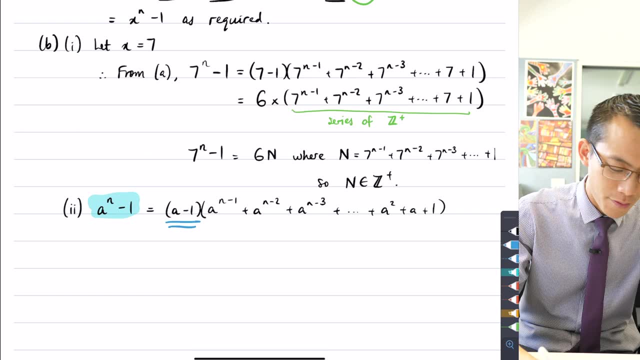 this thing gets bigger as a increases. so this part, this factor over here, this one can't be one, it has to be this: this has to be equal to one. so therefore, for a to the n minus one to be prime, oops, that minus one should be down here.